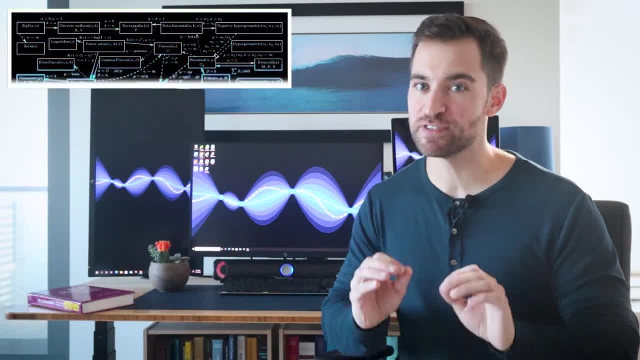 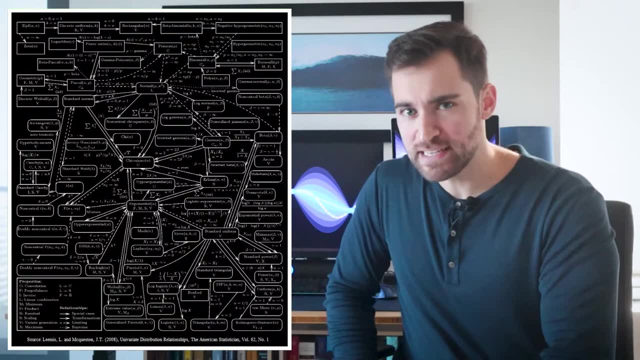 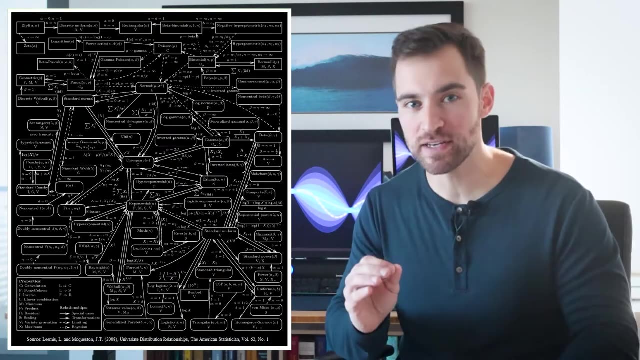 definitions Now, because the world of probability distributions, their properties and their relationships is huge, the compressed pattern that relates them is still quite big. Compression helps. If you want such a huge, valuable bag of information, you still must pay with focus, time and patience. 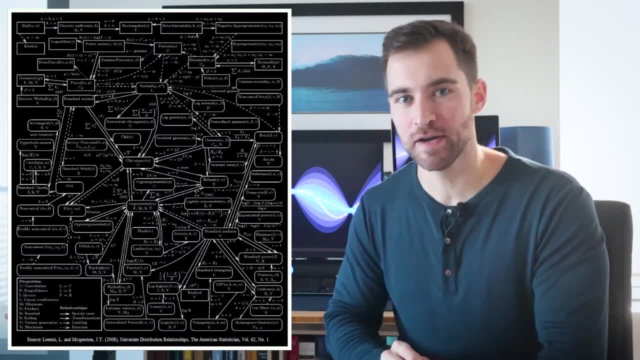 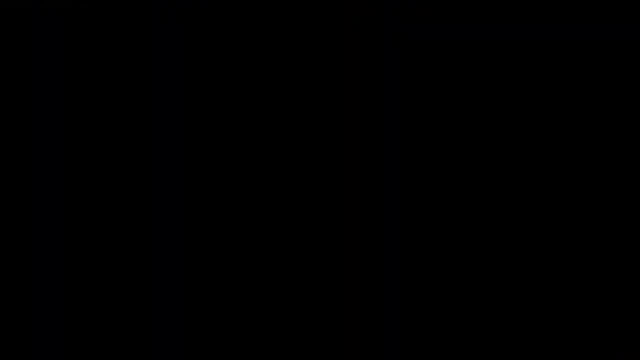 And if you're curious about this graphic, more on it at the end. But for now I'll start by telling you one of these stories that relates six of these distributions. We'll start with the simplest of random variables, the Bernoulli, One sample of this. 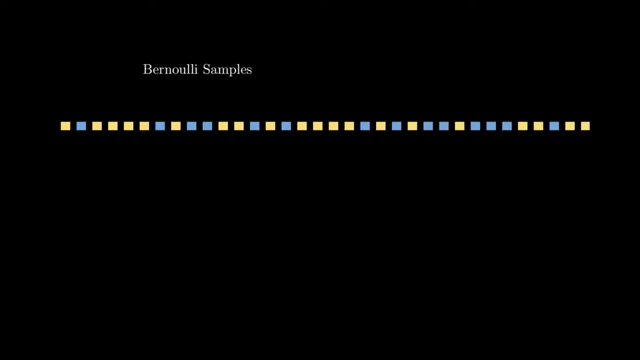 guy yields one of two outcomes: either yellow or blue. It has only one parameter, the probability of a blue box, which I'm writing here as p, and I've chosen specifically to be 0.3.. Now let's measure these boxes to produce another random variable. Specifically, let's 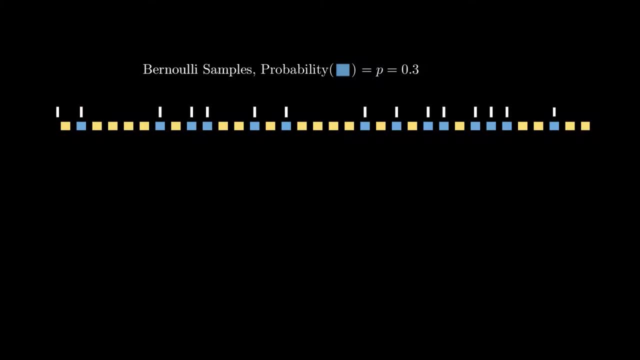 draw lines above each blue box and count the yellow boxes between them. The punchline is: this list of numbers would have a geometric distribution and it carries the same parameterization as our Bernoulli, which is that number p. Not too bad so far. 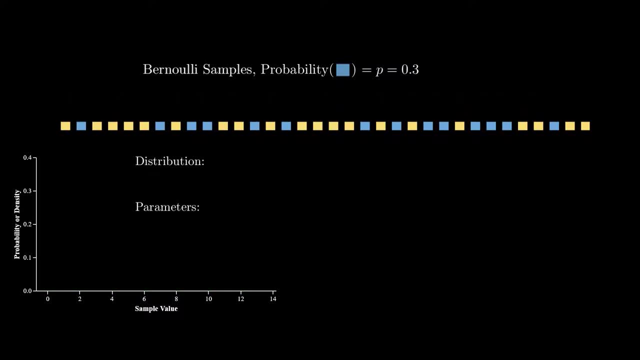 Next, let's apply a different criteria for those lines. Let's draw one over every other blue box and count the yellow boxes between those. Well, that would give us the negative binomial distribution with its r-parameter equal to 2.. If we picked every third blue box, the r-parameter would be 3.. Alright, still not. 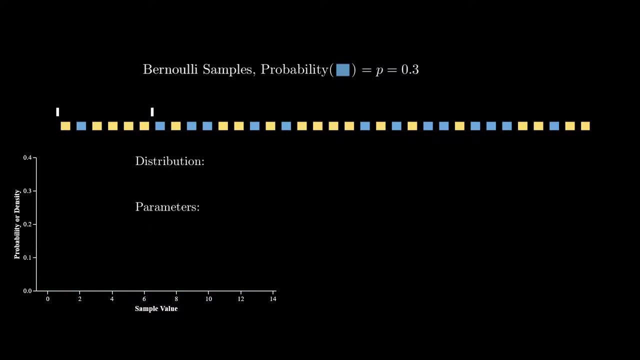 too bad, Let's try another. Let's draw lines separating groups of six boxes and count the blue boxes between those. Well, that would give us the binomial distribution, with its n-parameter equal to 6.. Hopefully you're getting a sense for how these distributions are similar. They're all. 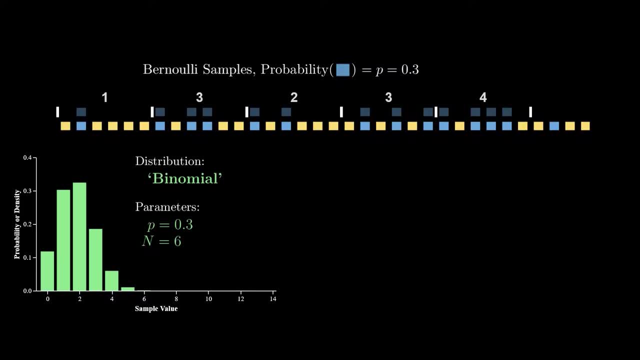 measuring the same thing, but with a different criteria for counting. So let's step it up a bit. Let's try to make a continuous version of these boxes. One way to do that is divide the probability of a blue box by some large positive number, c, and make each box count. 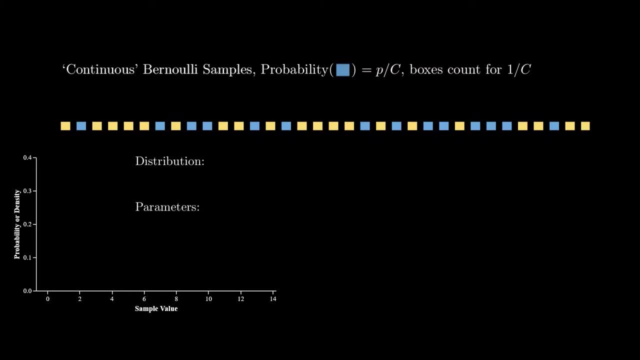 for 1 over c instead of 1.. As you can probably guess, I'd like you to pretend this number c approaches infinity, But that's not going to happen. You're going to have to do something about that. But to keep things tame on screen, I'll go with c equal to 5.. 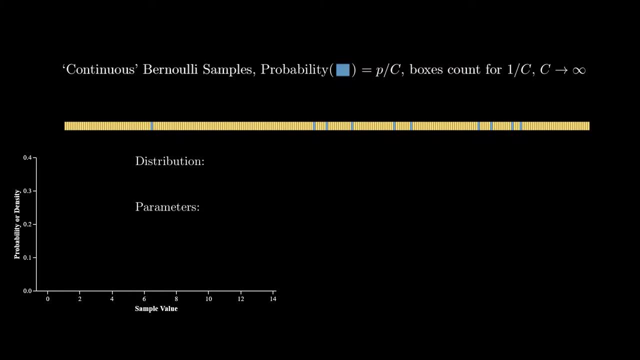 With that, let's reapply our previous criteria and see what we get. If we were to sum the boxes between all blue boxes, keeping in mind that each box now counts for 1 over c, then those numbers would be exponentially distributed. The r-parameter. 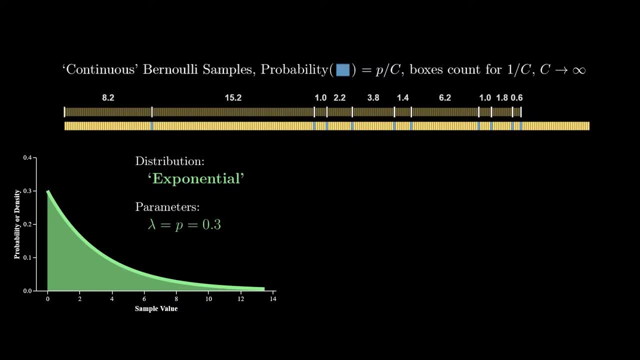 in this case would be p. I should note, the r-parameter is not p over c, which in the limit would be 0. But rather it's p, the probability of a blue box in this case. So we're going to sum the blue box in the discrete case we just came from. 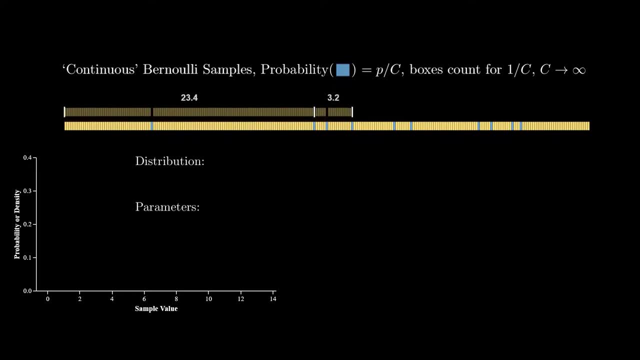 Moving on. if you were to sum the boxes between every other blue box, then you would get a gamma distribution with the shape parameter equal to 2 and the scale parameter equal to 1 over p. As you can see, the gamma distribution can be viewed as a continuous version and. 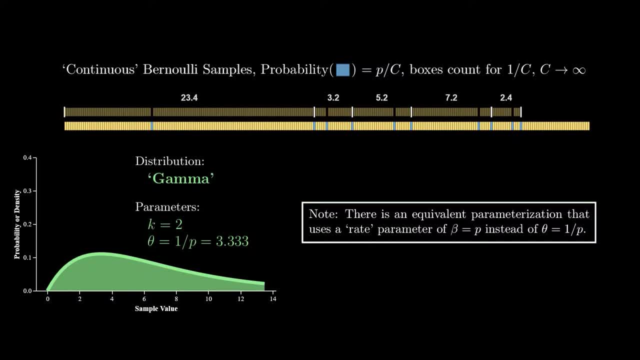 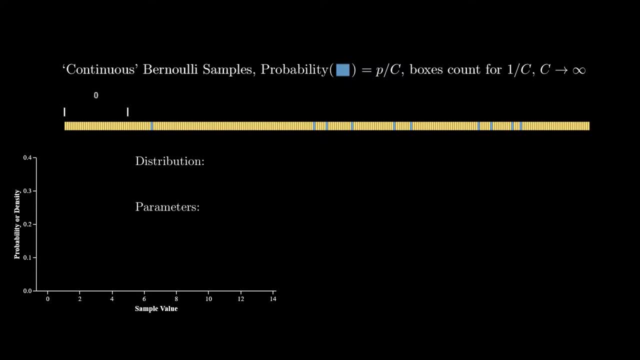 in fact a generalization of the negative binomial. Alright, last one. If you were to count the blue boxes between each block which sums to 6, then you would have a Poisson distribution with a r-parameter equal to 6p. Who saw that? 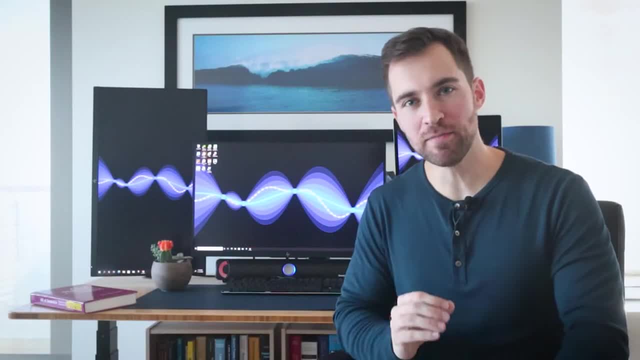 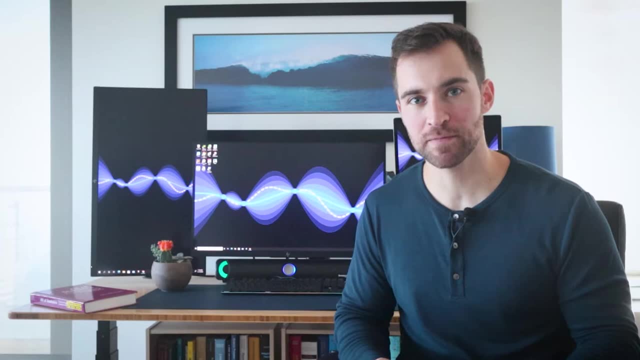 coming. Ok, let's take a step back. My argument is: if you want to understand these 6 distributions, you should focus on this short story. It's just good bang for your buck. It tells you a lot and it's not that hard to remember. In fact, I think I could cram it into this. 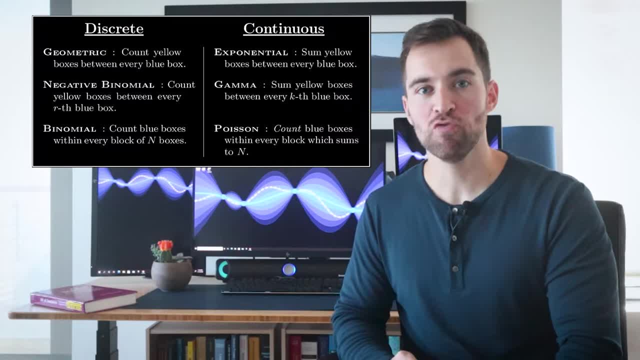 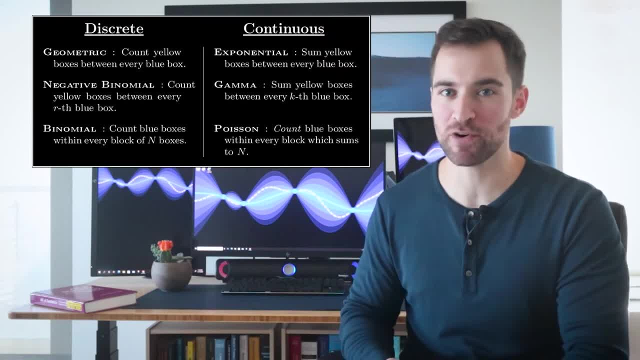 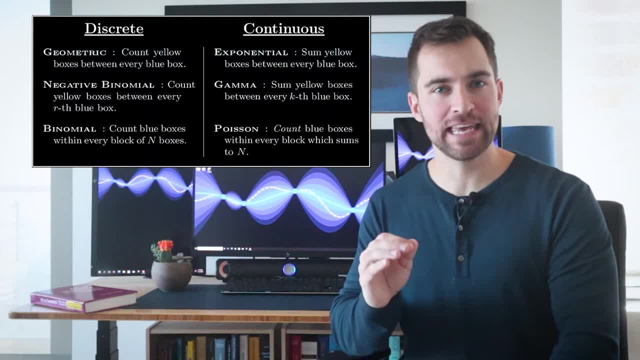 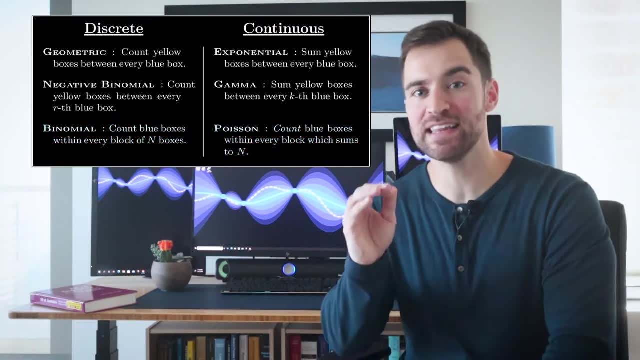 analogies: The exponential is the continuous version of Geometric. The Gamma is the continuous version of the negative binomial. The Poisson is the continuous version of Binomial. Also, I am putting the Poisson in the continuous section because it measures continuous things. 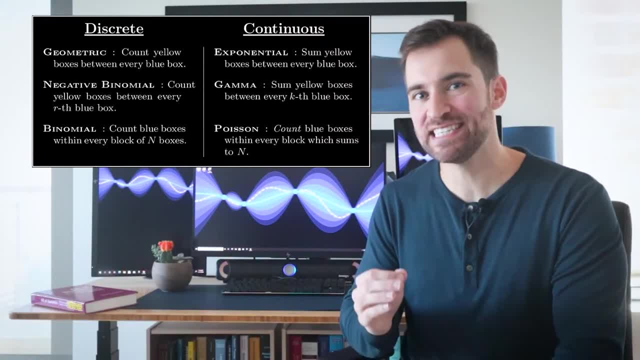 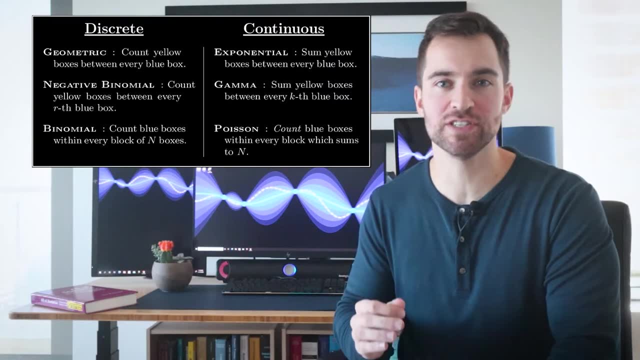 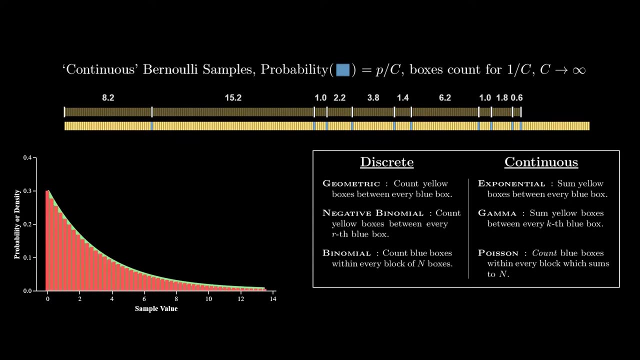 With that said, these analogies are useful In my experience. continuous distributions can be hard to reason about. Their parameters just aren't interpretable, so we can reason with their discrete versions in their place. For example, I think of the exponential distribution as a geometric distribution with thin boxes. 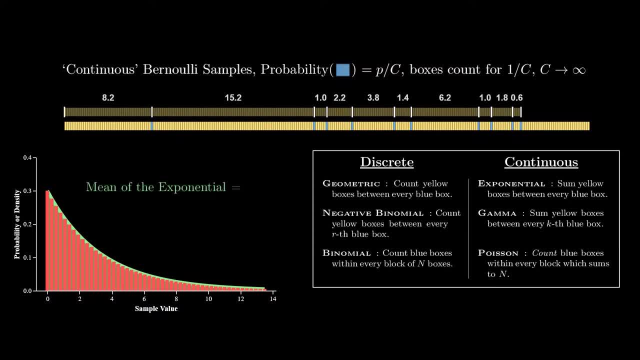 That's useful when trying to remember things like the mean of the exponential. The mean of the geometric is easy. it's 1 over p Meaning. if a blue box shows up 10% of the time, then on average I have to observe 10. 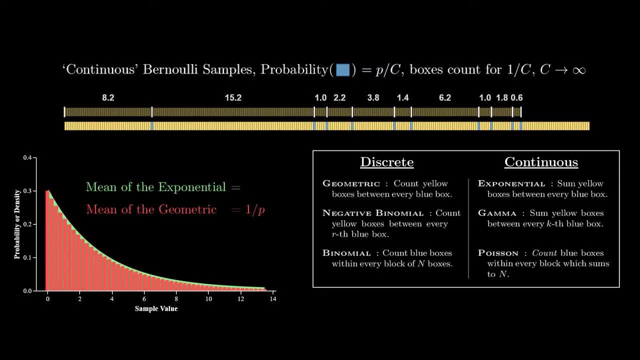 boxes before I see my first blue box. Okay, what about the exponential? Well, by analogy, it must also be 1 over p or, after you do the parameter translation, 1 over lambda. See how this can be helpful. And clearly, this sort of moment translation doesn't stop with the mean of the exponential. 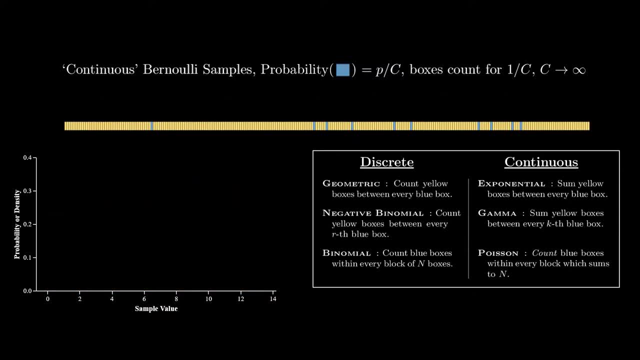 though that may be the simplest one. The next pattern to notice is the summation relationships. That is, if you sum samples of the geometric, you get the negative binomial, and, by analogy, if you sum up the exponential, you get the gamma. 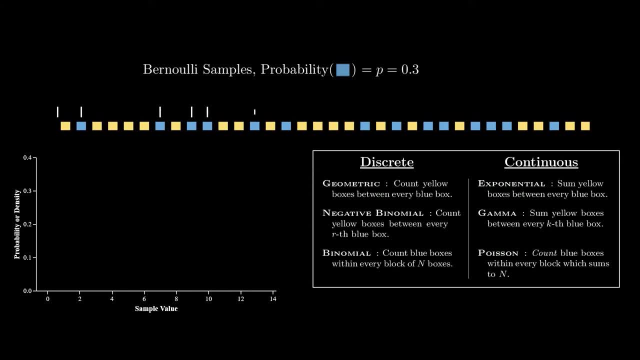 To see that. let's revisit those separating lines above. Now, if you wanted to show the sum of two geometrics with this view, how might you do that? Well, since we know the geometric is just the number of yellow boxes between lines. 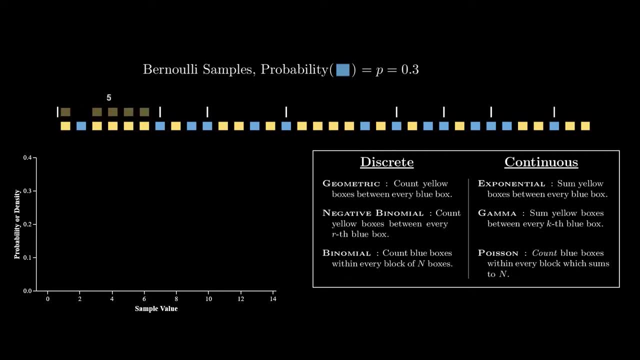 we could drop every other line and then count between the remaining lines, But notice, these are exactly the same separating lines of the negative binomial with r equal to 2.. So we see, summing up, geometrics gives us a negative binomial and, by analogy, the same. 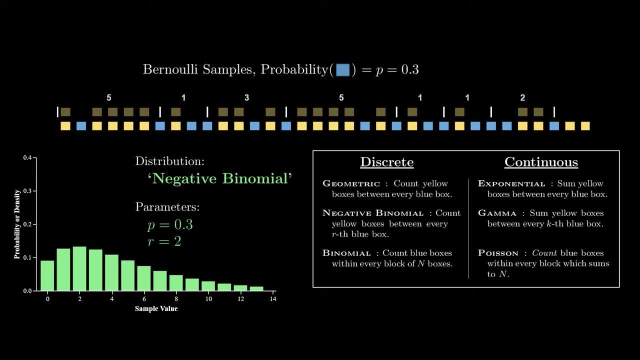 argument shows that the gamma is a sum of exponentials. Now, that is insight. And in fact you could use a similar argument to show that summing up binomials yields another binomial, And the same is true for a Poisson. 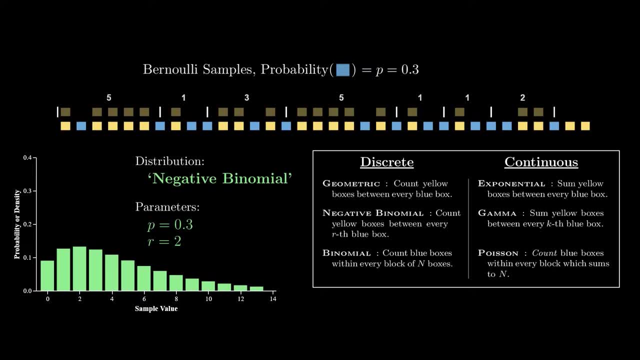 It would be pretty easy to figure out their parameters too. And if you smuggled in the central limit theorem, that tells you why four of these distributions approach the normal distribution as some select parameters become large. More insight, So hopefully that convinces you. It's easier to understand the Crowder theorem than it is to understand the Poisson theorem. It's easier to understand the Crowder theorem than it is to understand the Poisson theorem. It's easier to understand the Crowder theorem than it is to understand the Poisson theorem. 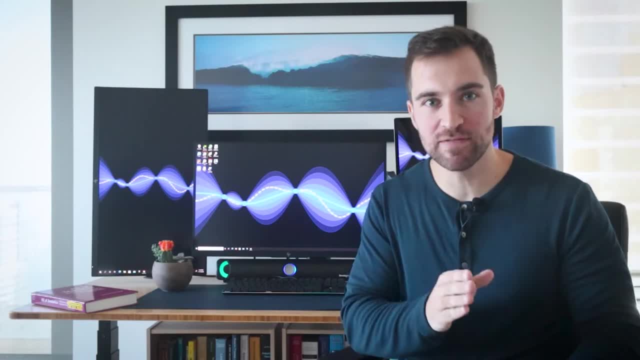 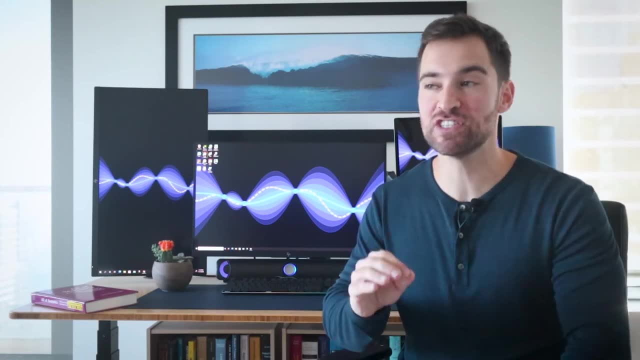 The Poisson theorem is a formula of distributions, if you remember the stories that relate them rather than their individual definitions. And that's because those stories offer additional properties virtually for free, And those crystalize the whole picture and burn it into your brain. 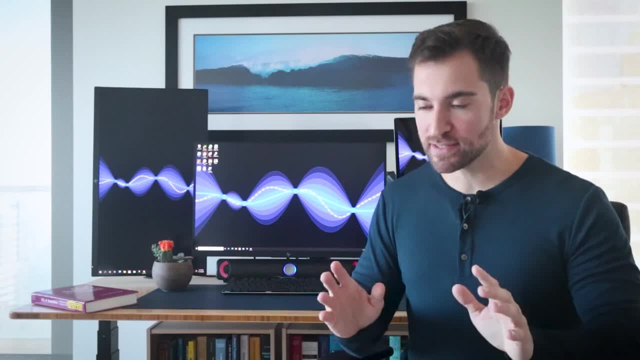 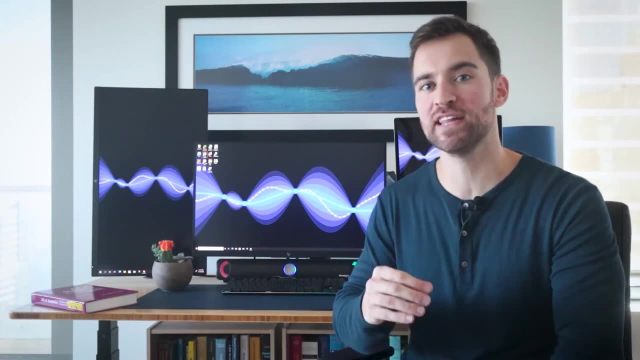 But, as you may have noticed, that hardly covers everything. Well, yes, the compression ratio, at least from what I can see, isn't as dramatic as we may hope. There is some fragmentation of stories, each of which only relates a handful of distributions. 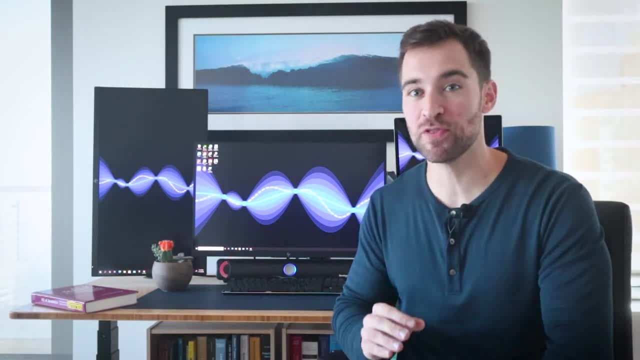 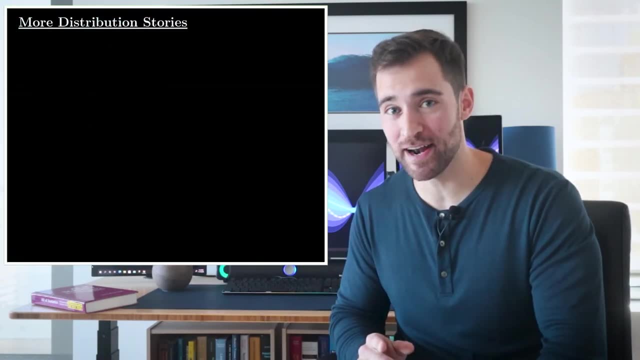 Still, those are worth remembering. That said some of the range of these stories, I'd like to quickly fire off a few of my favorites, just as a bonus. Ready, I'm about to throw a lot at you. Okay, say v is just some fixed positive number and you have a gamma distribution with both. 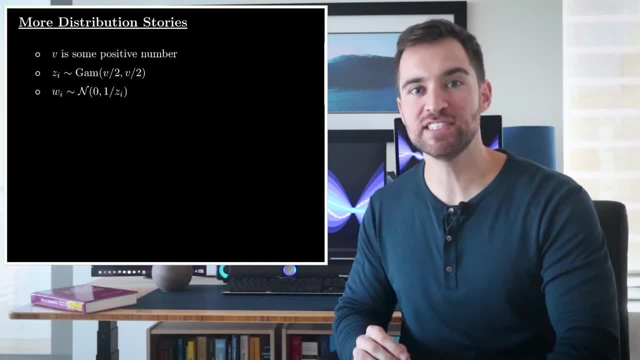 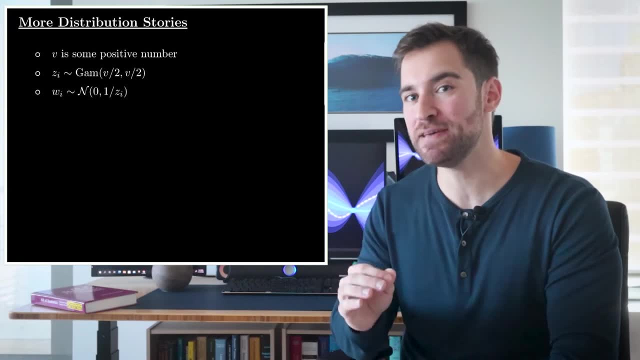 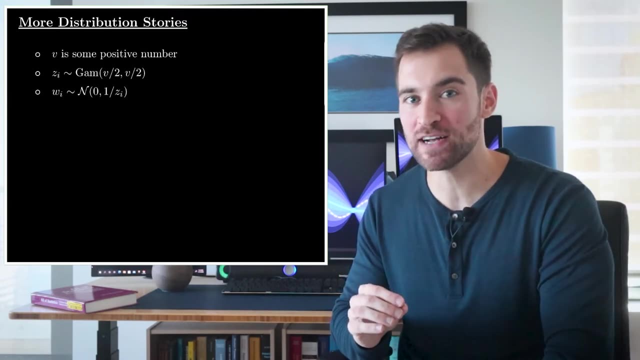 its parameters set to half of v. Then you sample from that gamma some value which I'll call zi. Then you use 1 over zi as the variance in a mean-zero normal distribution, And then you sample a value from that which I'll call wi. Well, if you repeated that process, 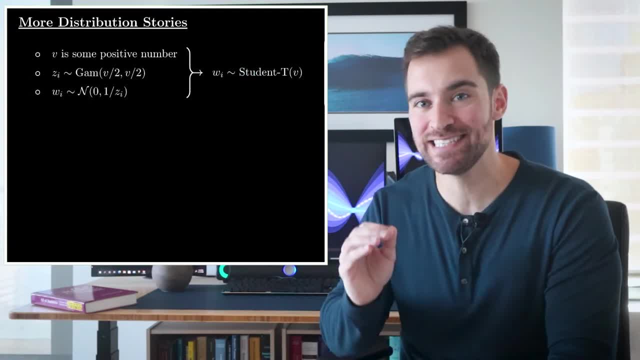 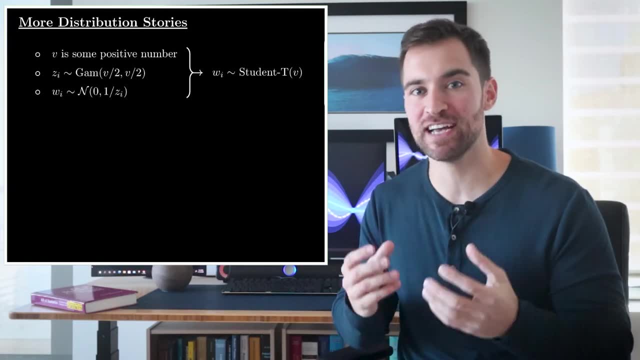 many times, you'd discover that wi has a student t distribution with v degrees of freedom. I'm not sure why, but it was only when I learned that fact that I started to get comfortable with the student t distribution. The student t is just a bunch of normal distributions. 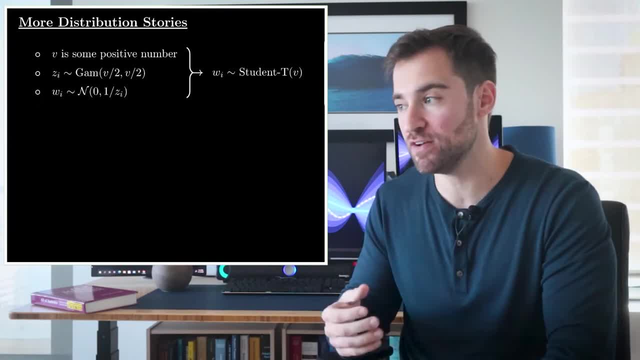 mixed together with different variances that bounce around according to an inverse gamma distribution. Okay, another, Let's say we have an exponential distribution with some fixed lambda values, Then you sample a value from that which I'll call wi. Well, if you 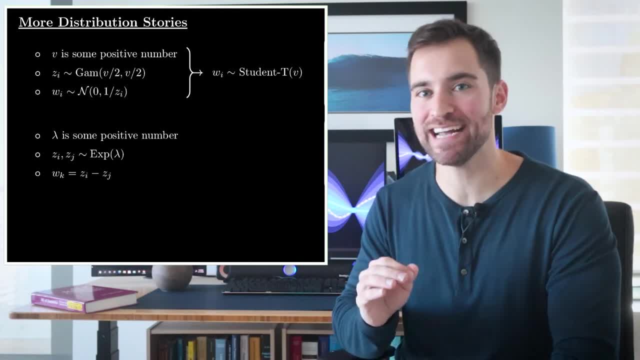 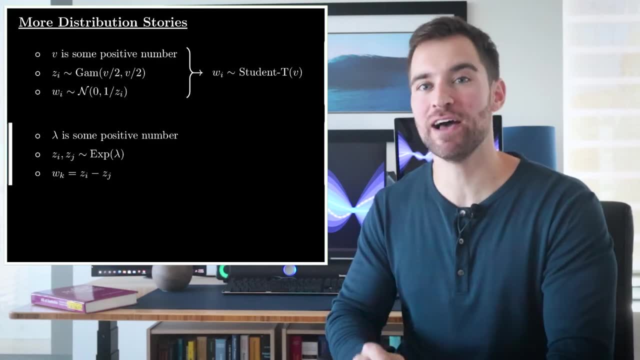 parameter. We'll draw two samples from that exponential, zi and zj, and take their difference and call that difference wk. Well, in this case wk would have a Laplace distribution. If you don't know about the Laplace, it shows up a lot in machine learning for generating sparse. 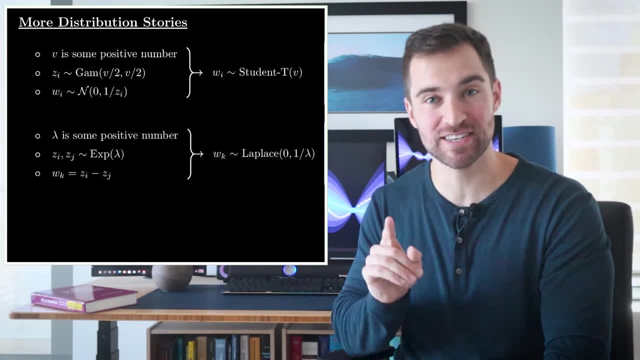 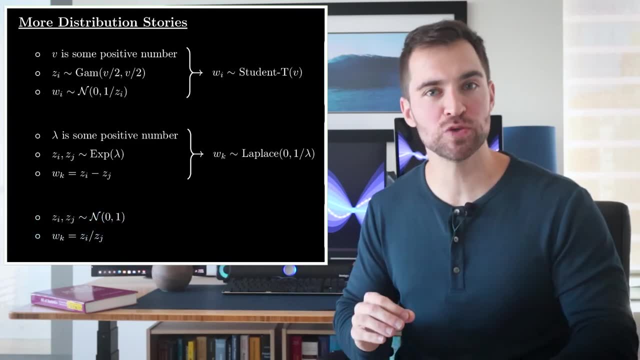 solutions. And again, I felt it was pretty unintuitive until I saw this angle. Okay, last one. Let's say we sample two values from the standard normal distribution again, which we'll call zi and zj. Then let's say wk is their ratio. Well, in this case, 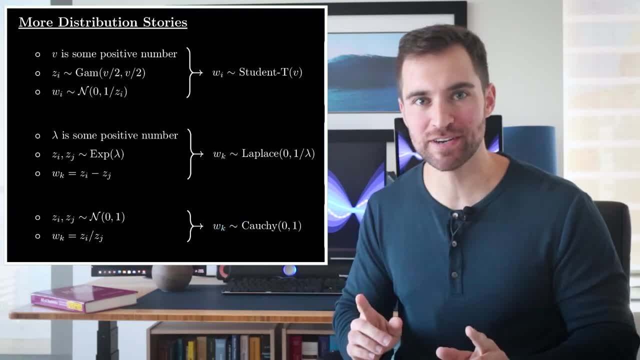 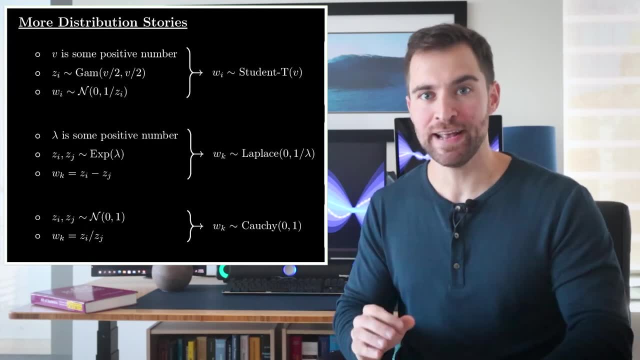 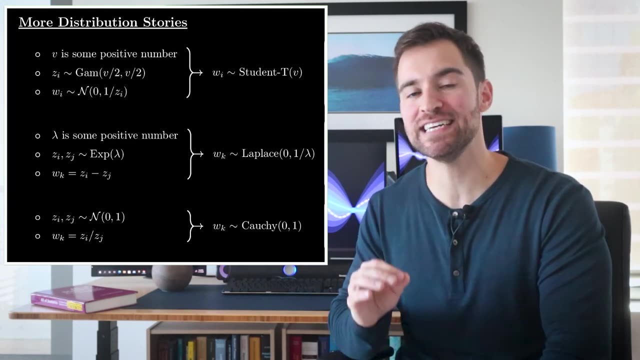 wk has a Cauchy distribution. Excuse my redundancy, but again this demystified the Cauchy distribution for me a lot. The Cauchy distribution is weird. It has an undefined mean and variance which I felt made no sense. But it made a little sense after I realized it's a ratio.